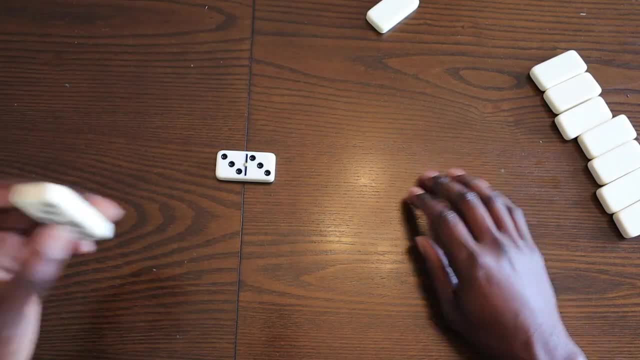 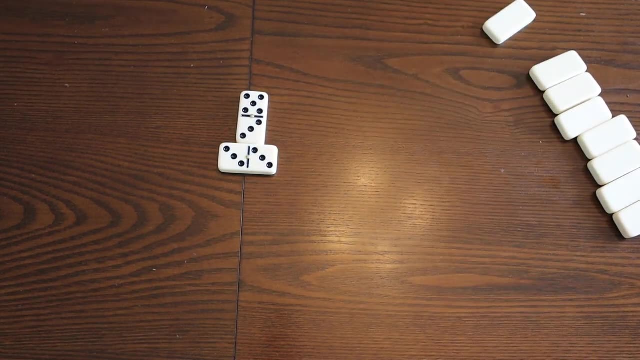 So they got to go to the boneyard and pull and they, what do they come out with? They come out with tray five. So now, what do you do in this instance, when they have tray five? Well, what you do is you immediately hit that five. 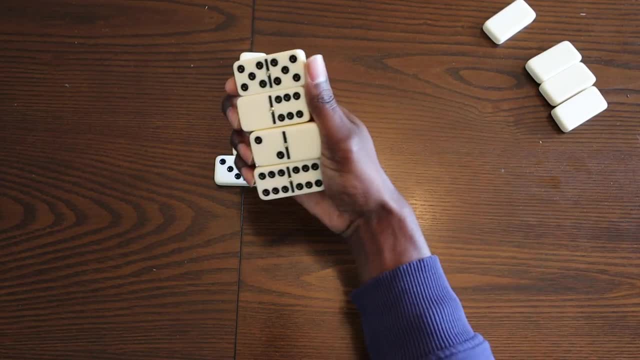 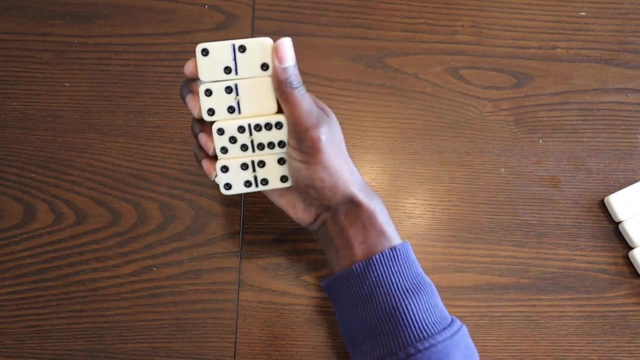 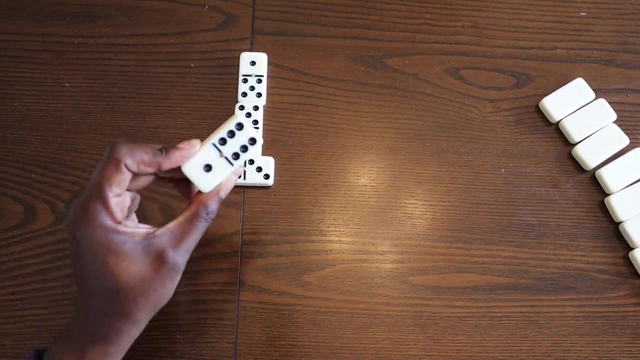 Now it's back on the opponent. So we look into their hand. We know they're not touching the tray. Do they have an ace? They got no aces either, So they're going back to the boneyard again. What do they come out with? They come out with ace six. 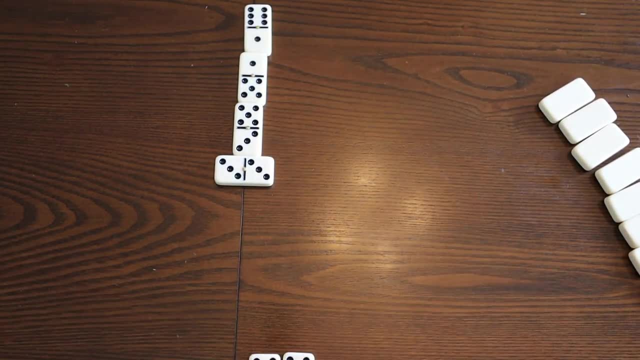 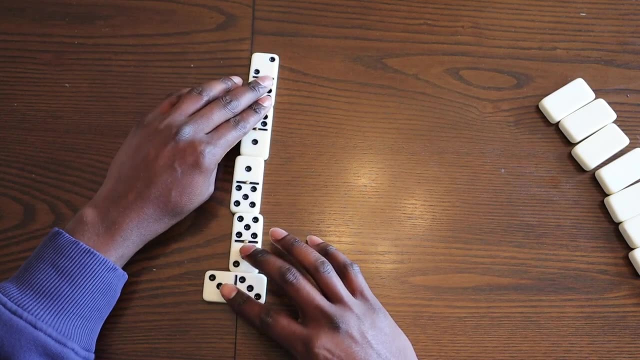 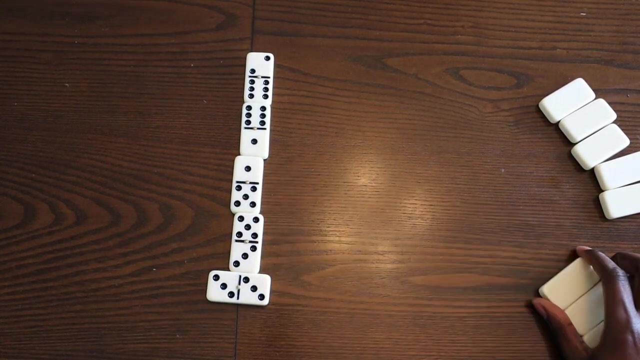 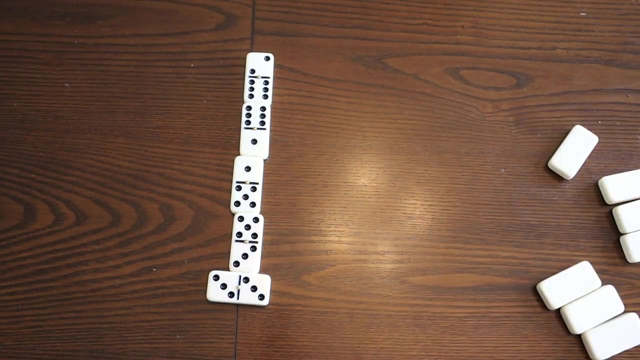 They put a six up Now in our hand, what do we do? Of course we want to chop that six down right away. Let me move this back into the frame for you guys. Of course we chop that six down right away. We look into their hand here. Most of the time, the average player they could either play the 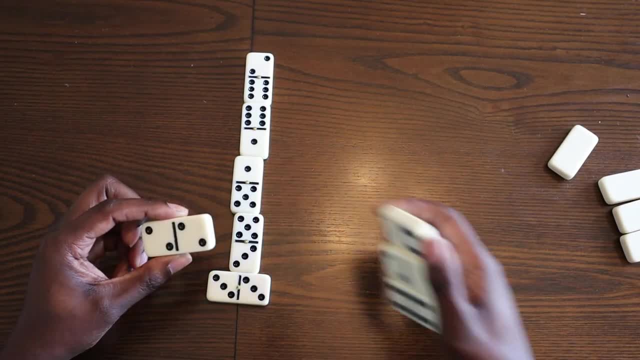 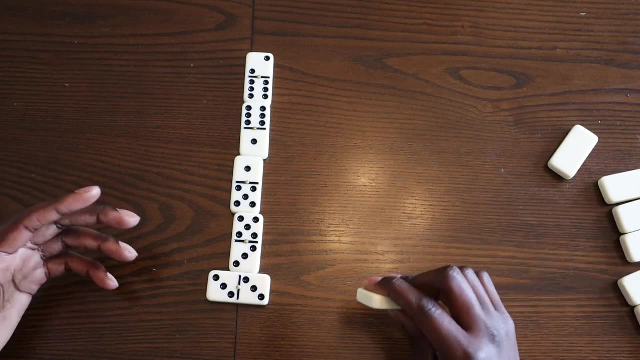 deuce, blank or the double deuce. The average player is always going to shoot for the double deuce. Why? Because they want to score. They know they're behind, They have so many dominoes in their hand and this is when they 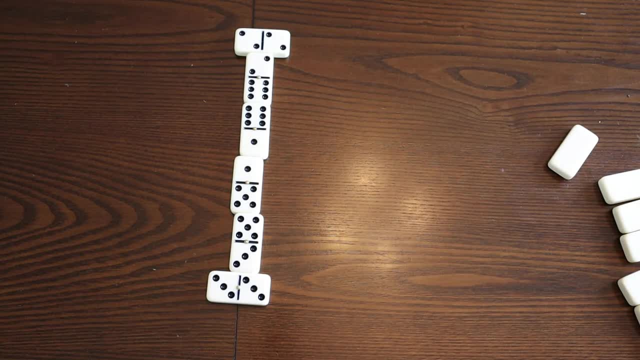 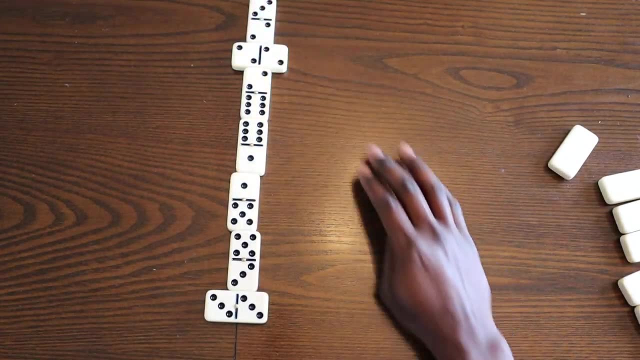 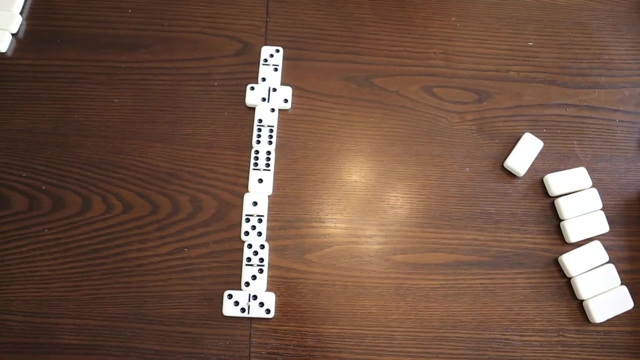 come with the double deuce and they would count ten. Now that is a nightmare for them, because at that point, that's when we go hard with the deuce tray And where do we send them? Right back to the boneyard again. So they're going back to the. 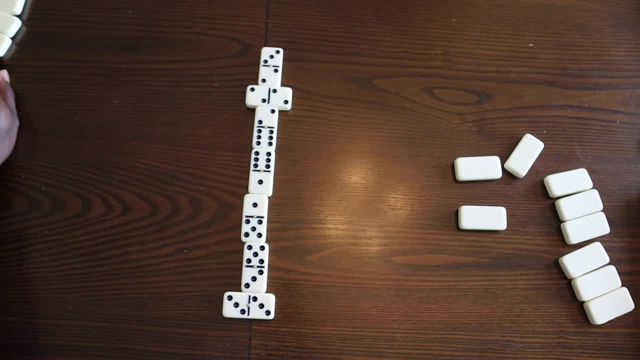 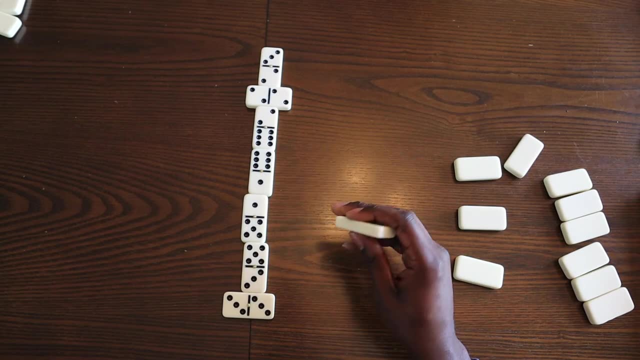 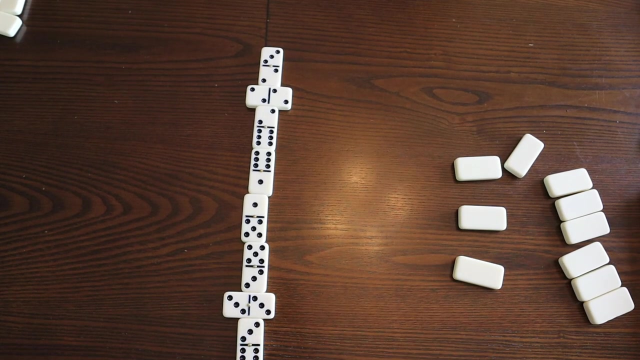 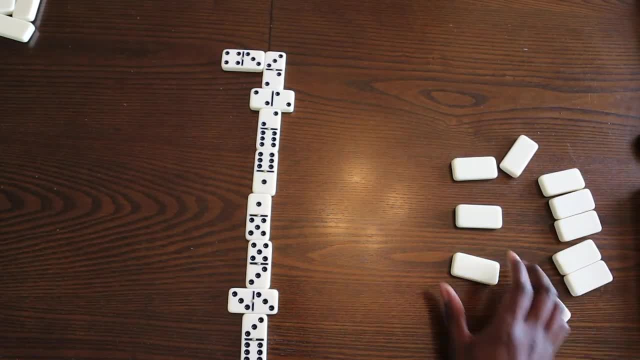 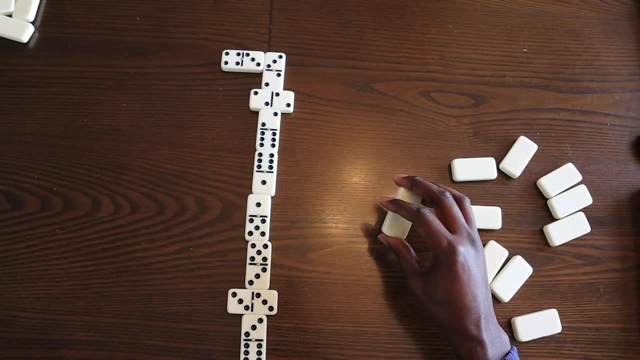 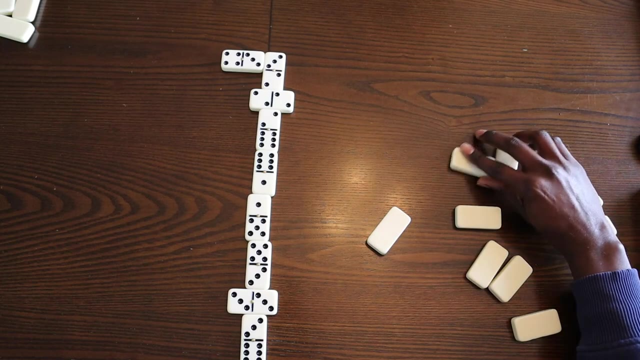 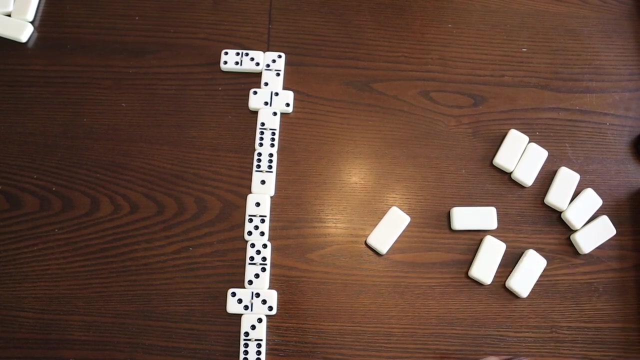 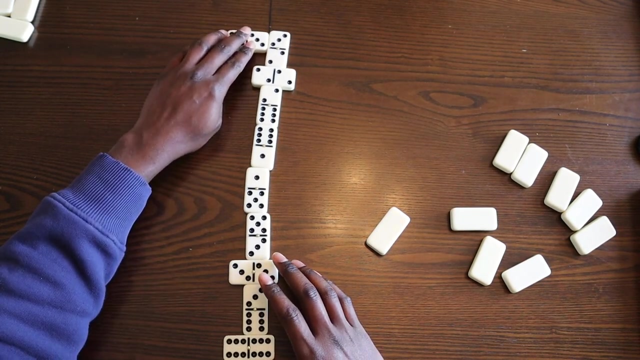 Angle that. And then the next thing that they can do, they could either play the double four, double six- Let's say they drop the double six there. So then now we're running for the border A little bit, A little bit at this point, because we don't have